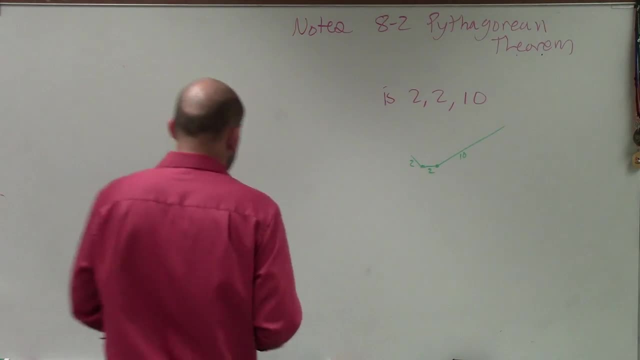 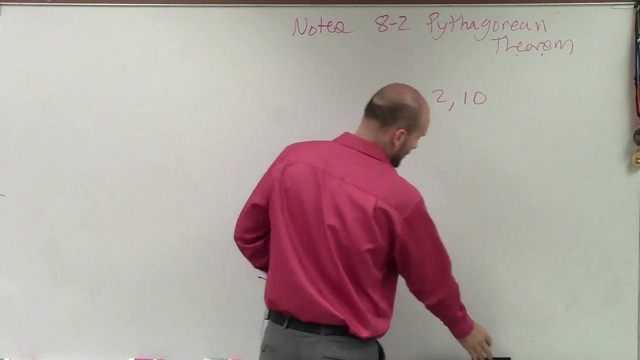 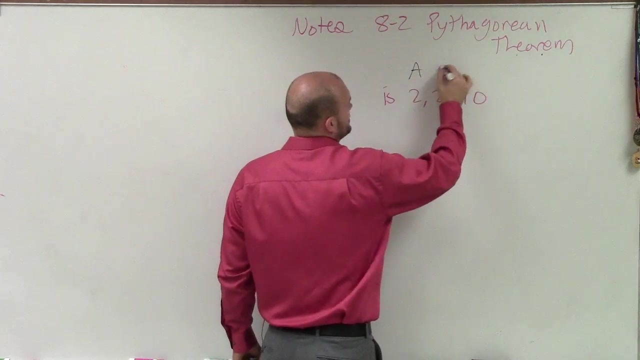 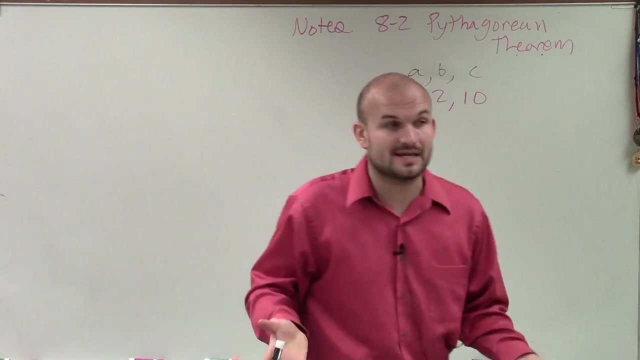 So what we're going to be talking about, guys, is we're just going to be talking about determining if three side lengths create a triangle. alright, And what I want to show you, guys, is by using this inequality to determine if three side lengths create a triangle. we're going to look at- let's call this length A- B, let's do lowercase A, B and C. alright, If you have side lengths that create a triangle, you have to have the sum of two of the sides. 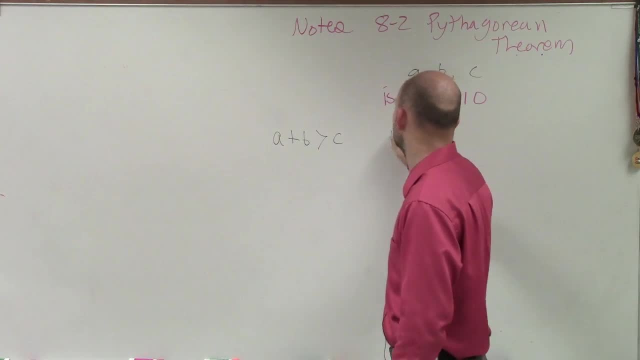 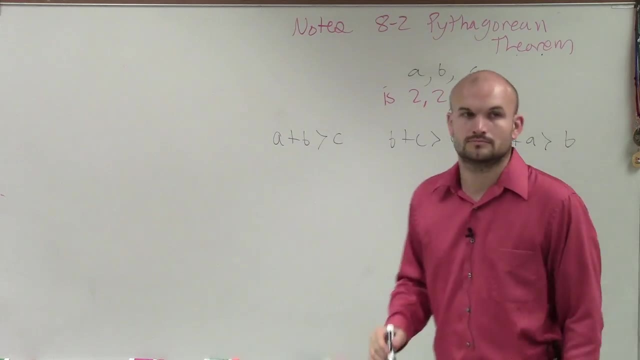 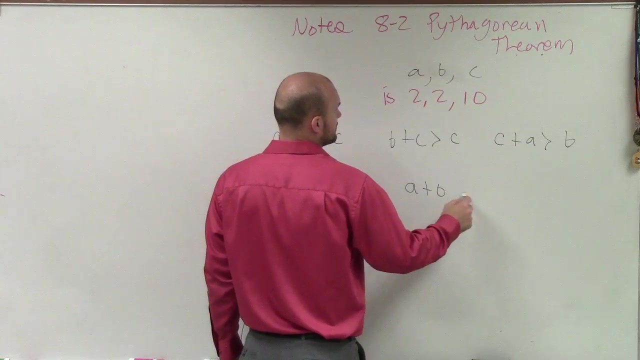 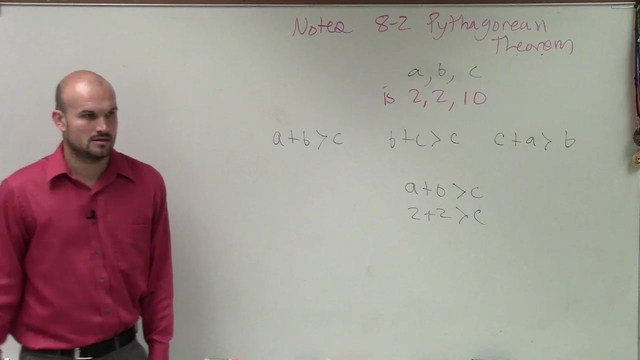 have to be greater than the third side. okay, And you guys can see that in this case, A plus B has to be greater than C. Well, is 2 plus 2 greater than C? Yes, Oh, I'm sorry. Well, is 2 plus 2 greater than 10? Sorry. 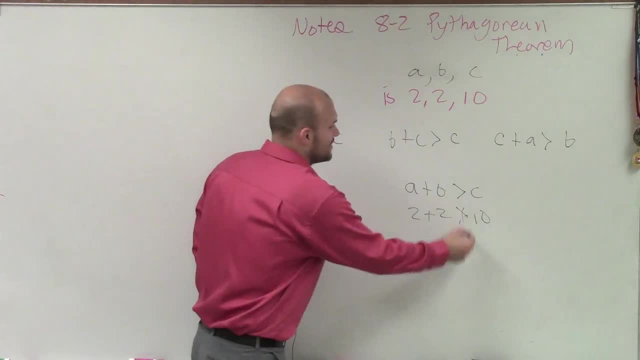 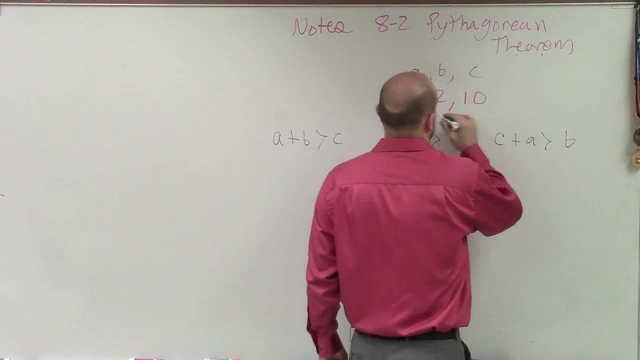 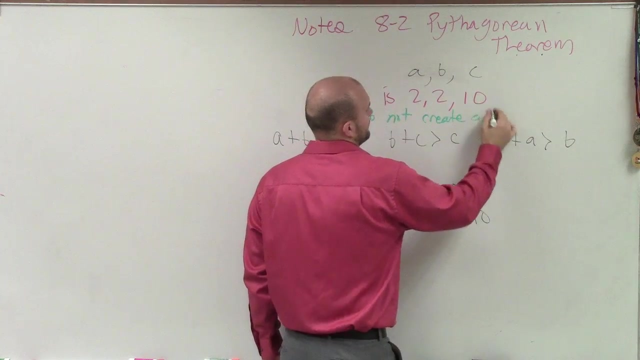 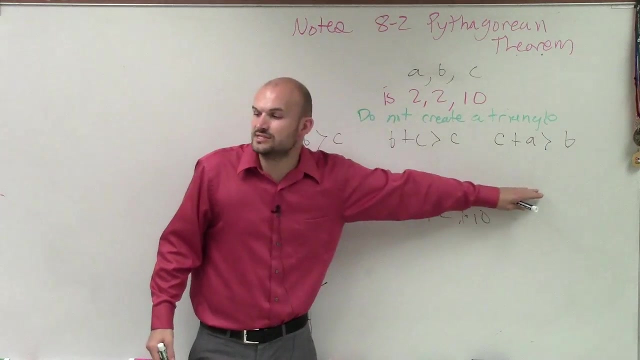 No, No. So therefore, that's incorrect. Therefore, these three side lengths do not create a triangle, alright, So you guys are going to want to make sure you have this written down so you can go back to the plot. that sum of two sides and measure have to be greater than the third side. 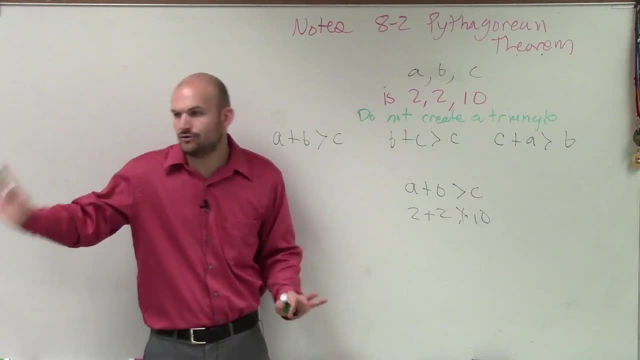 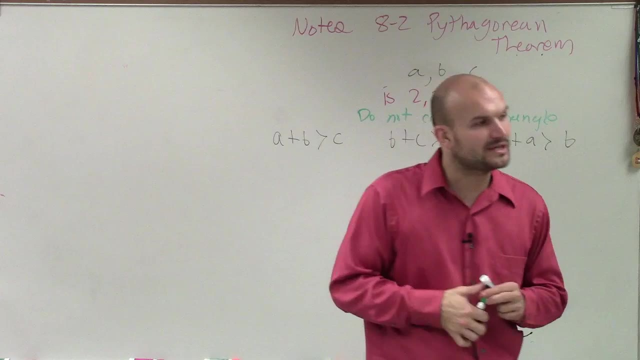 I'm not talking about acute scalene equilateral right triangles, Pythagorean theorem. I'm not talking about that at all. I'm just saying, if I gave you three lengths for them to be a triangle, it has to pass through this, alright. So,